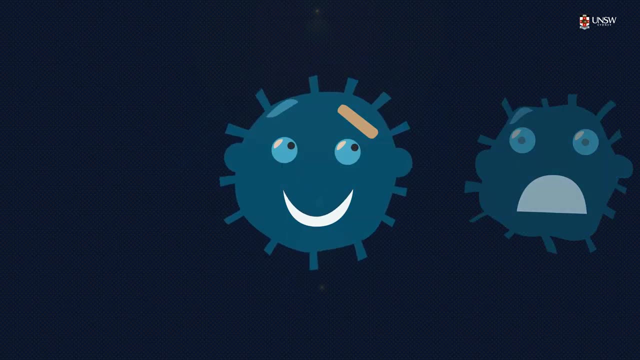 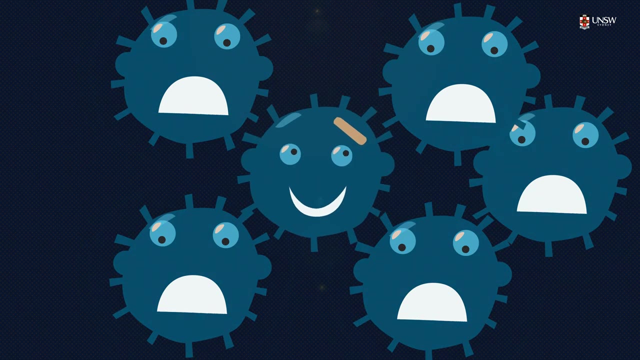 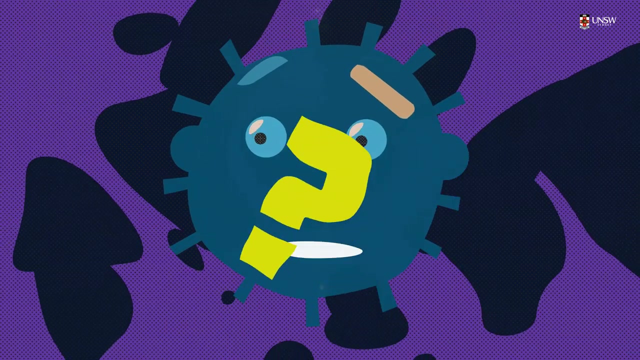 harmlessly, or it may repair itself. However, the third possibility is that it remains viable but produces with genetic errors, thus increasing the risk of cancer. Because radiation is potentially hazardous, the risk of using any nuclear technology is assessed against the ethical benefit. This justification is the first step in assessing nuclear safety. Take climate. 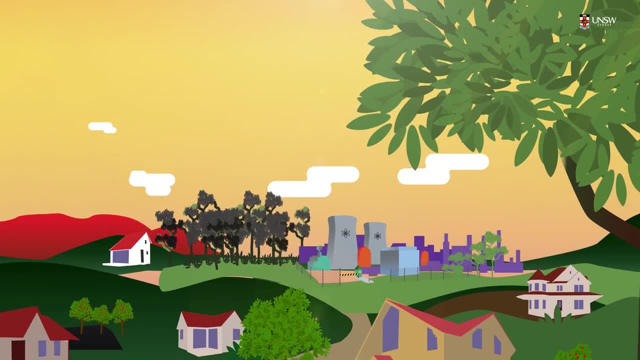 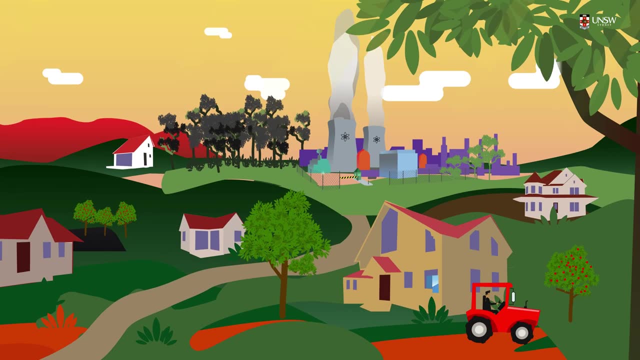 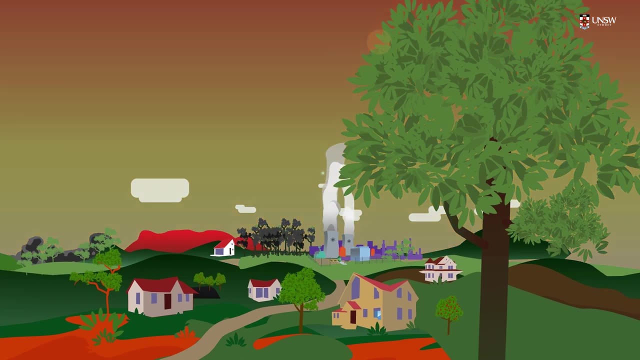 change, For tackling climate change while preserving biodiversity. there are strong benefits in nuclear technology. A working nuclear power plant is clean. Its power output is decoupled from the carbon cycle and is only weakly coupled to land usage. The high energy density fuel and reliable output provide energy. 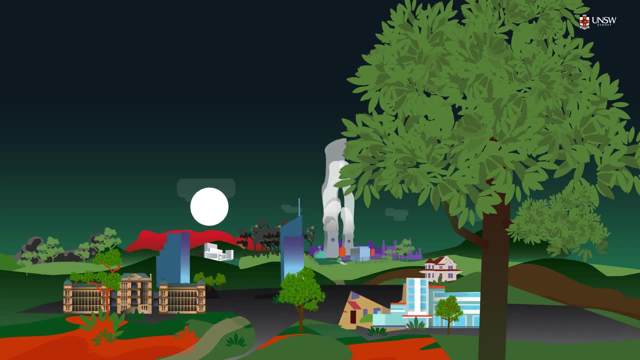 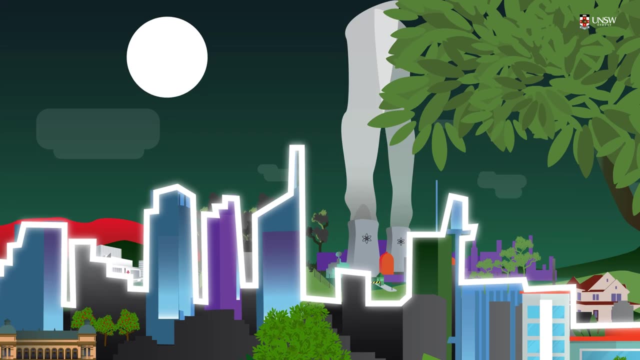 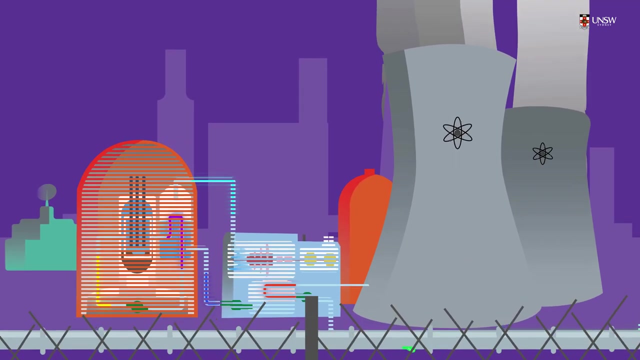 security to the countries that generate nuclear electricity. The waste is captured at the point of generation and has a very small volume, But irradiated nuclear fuel is unquestionably dangerous to living organisms. So any nuclear reactor comes with a risk of harming the people who offer. 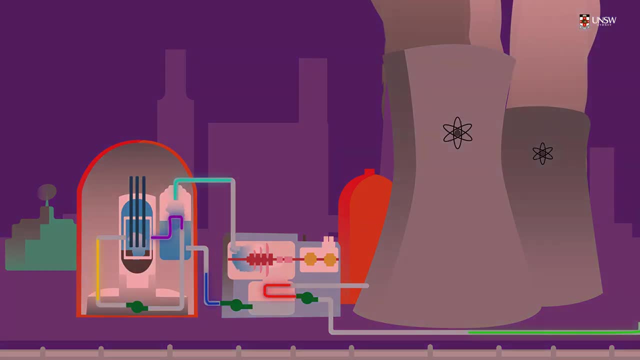 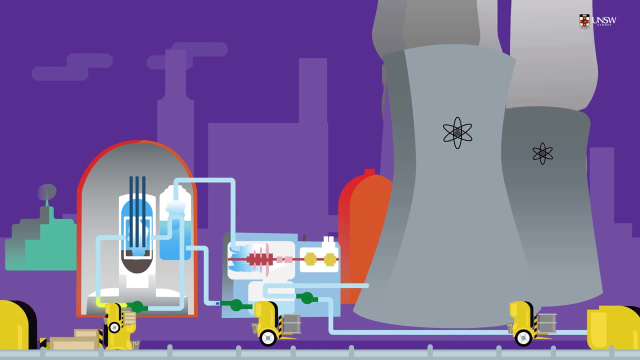 these nuclear facilities and the risk of harming the surrounding environment by releasing radiation. Because we understand how these risks originate and because we know how to control them, we justifiably opt for the benefits of using nuclear technology, and around the world, nuclear energy is used to provide energy. 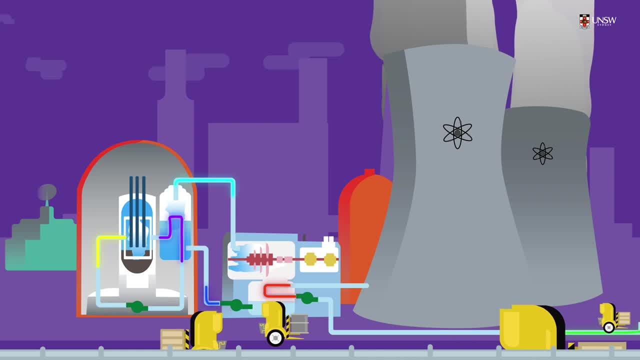 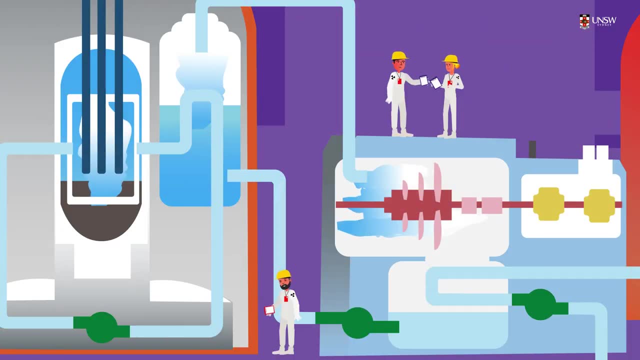 security while mitigating co2 emissions that would otherwise contribute to climate change. The full responsibility for safety rests with the engineers, That is, with us and the leaders of our organisations, Because, as engineers, we are the people responsible for facilities and activities that could give rise to significant radiation. 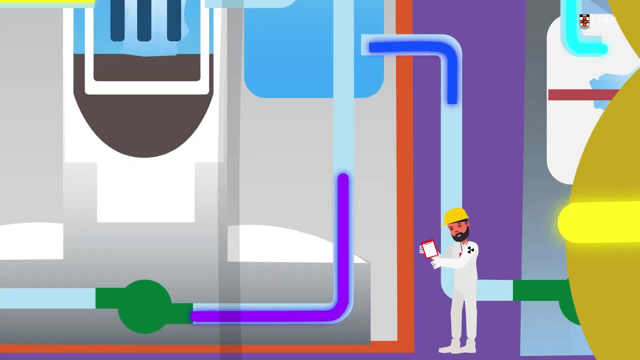 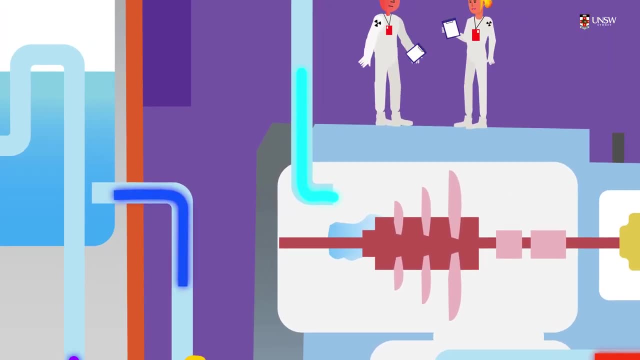 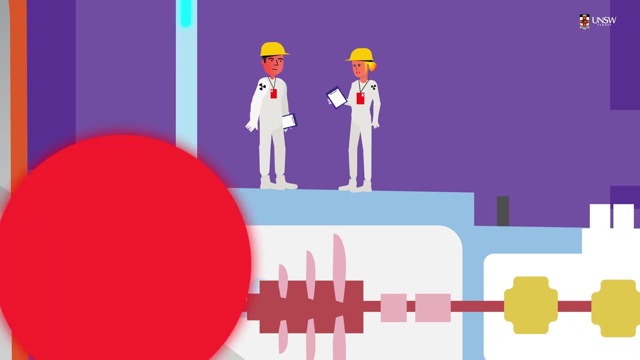 release To provide safety. we restrict the likelihood of events that might lead to a loss of control over a nuclear reactor, core, nuclear chain reaction, radioactive source or any other source of radiation. We prepare to mitigate the consequences of such events if they were to occur. 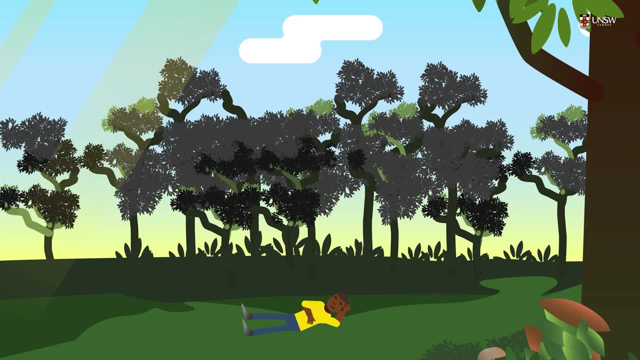 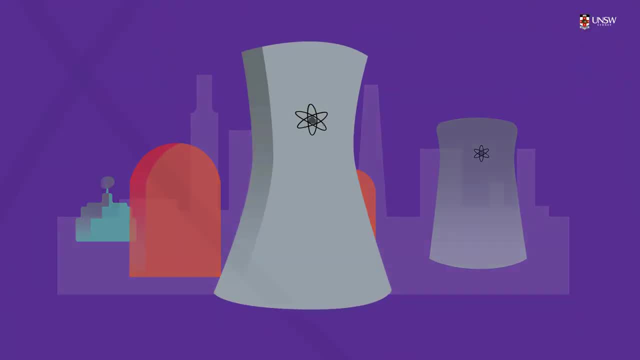 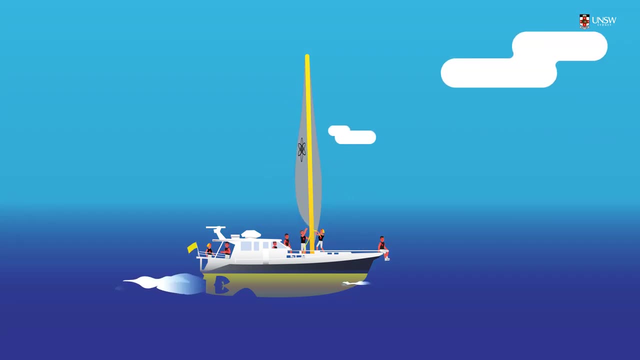 Both people and the environment, in the present and in the future, must be protected against radiation risks. This is challenging because the likelihood of serious accidents in a single nuclear facility must often be reduced to below chances of once in thousands of years, and no individual or automated system can achieve this. on. 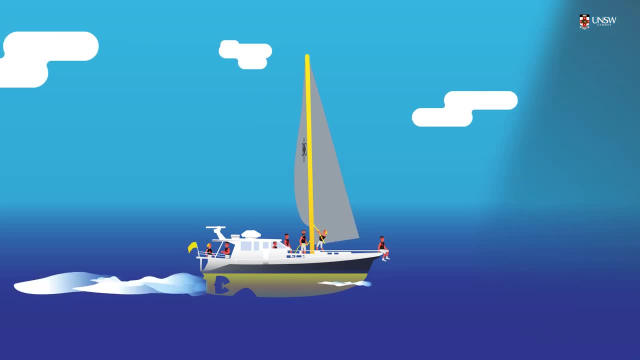 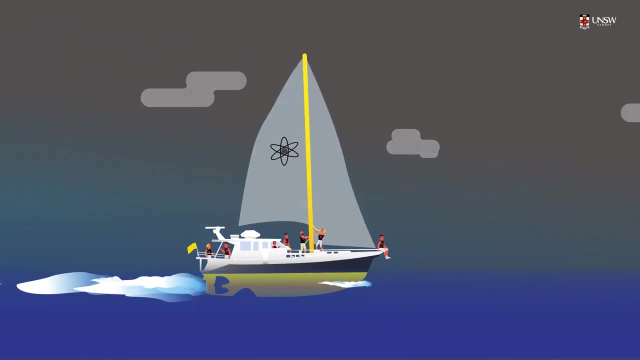 their own. Therefore, for the prevention of accidents, our primary measure is defence in depth. Properly implemented defence in depth ensures that no single technical, human or organisational failure could lead to harmful effects. Pursuing nuclear safety objectives, we make use of independent regulatory bodies, making these a part. 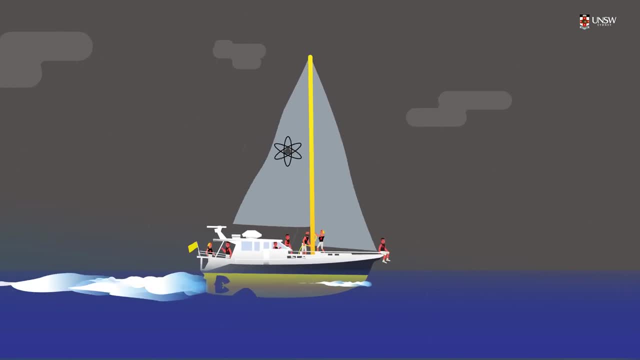 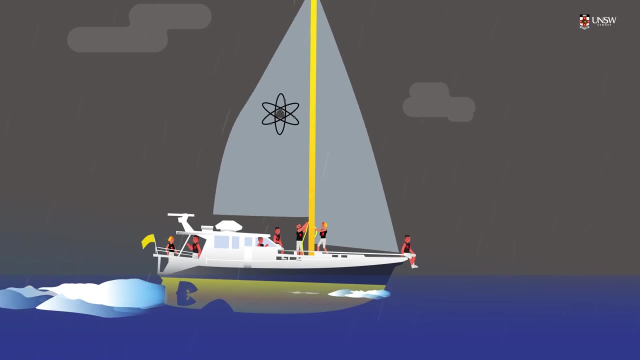 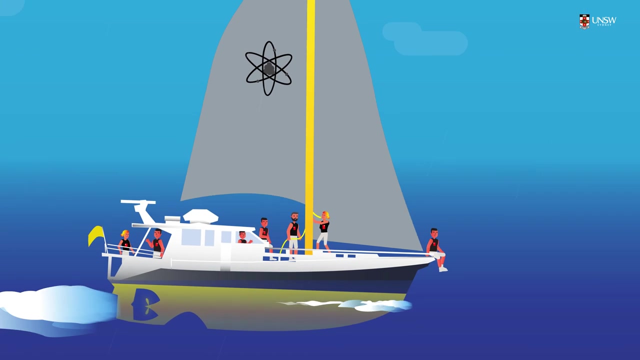 of the legal and governmental framework for safety in each of our states. We build structured organisations of individuals who work together, guided by principles of leadership and management for safety. With these factors, we ensure that we create the appropriate operational environments for highly reliable decision-making. The fundamental nuclear safety objective is to 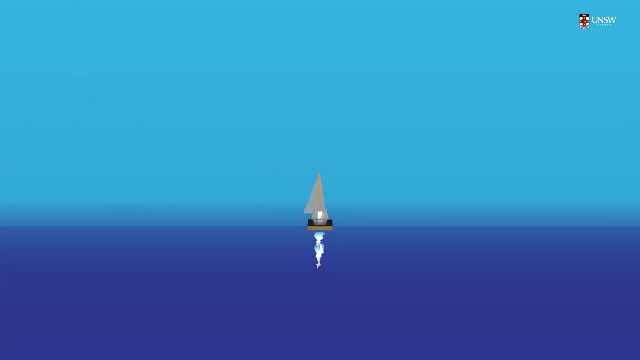 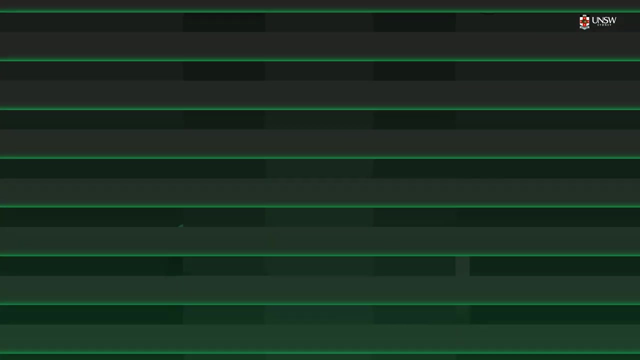 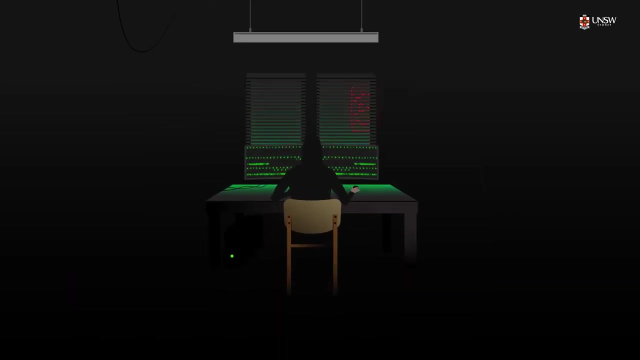 protect people and the environment from the harmful effects of ionising radiation. 2. Security: The need for nuclear security comes about because there are people with malicious intentions. Radioactive materials unavoidably form the target of some of these malicious intentions because they can be inherently dangerous if used in certain ways. 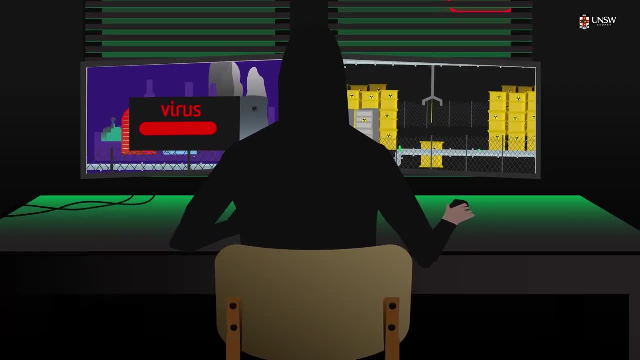 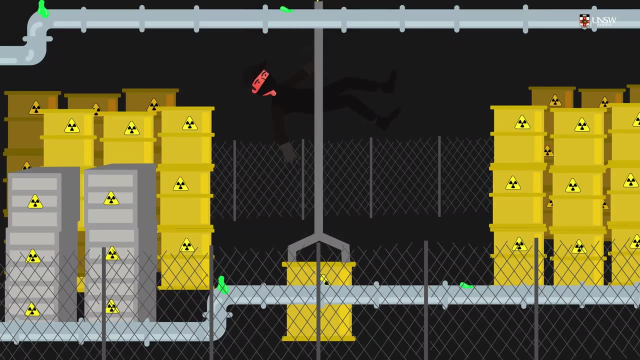 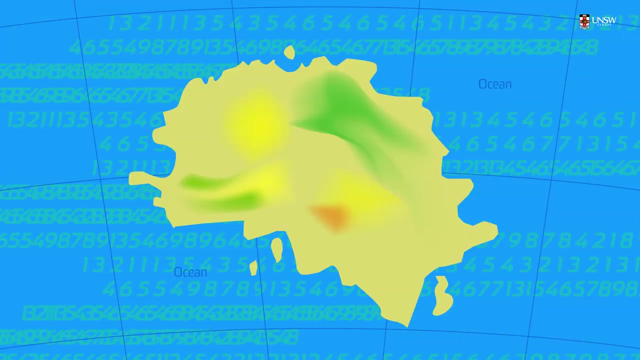 And because the illicit transfer in fissile nuclear materials may further the proliferation of nuclear weapons. Nuclear security, firstly, is the prevention of criminal or intentional unauthorised acts involving radioactive material, such as theft or sabotage. Ultimately, the state of jurisdiction for a nuclear facility is responsible for the security of its radioactive sources and nuclear 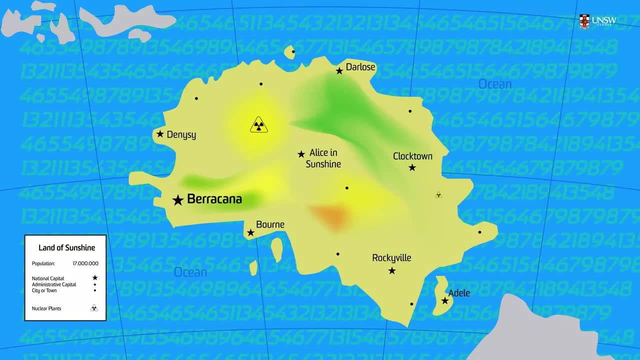 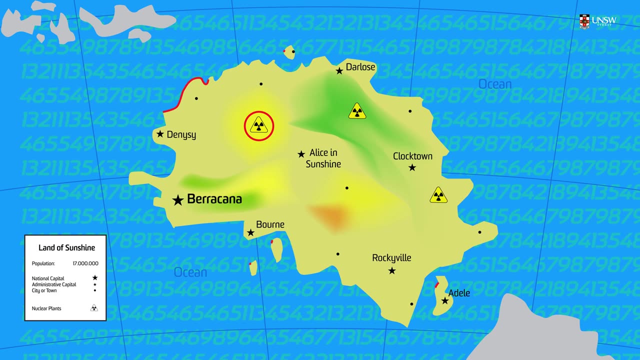 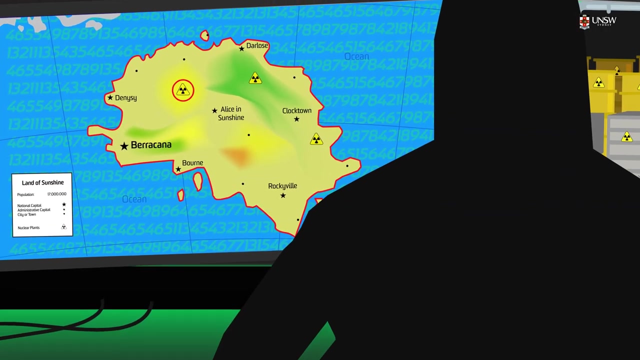 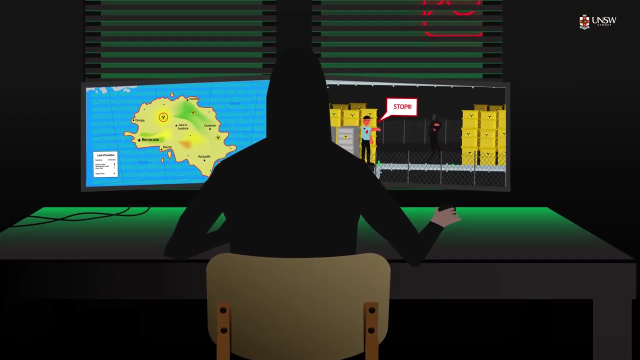 materials. The state maintains this responsibility To provide adequate protection during international transport of its radioactive sources and nuclear materials, All the way until responsibility is properly transferred to another state. Nuclear security includes preventing sabotage or malicious action against the nuclear facilities as well as the radioactive materials, as this could cause equal harm. An example would be: 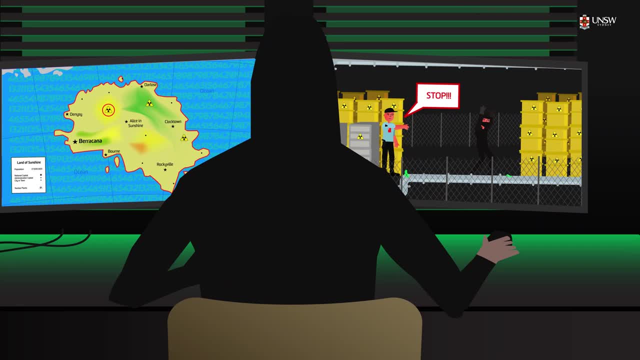 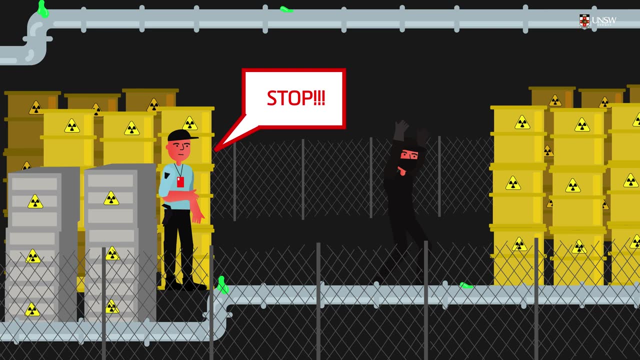 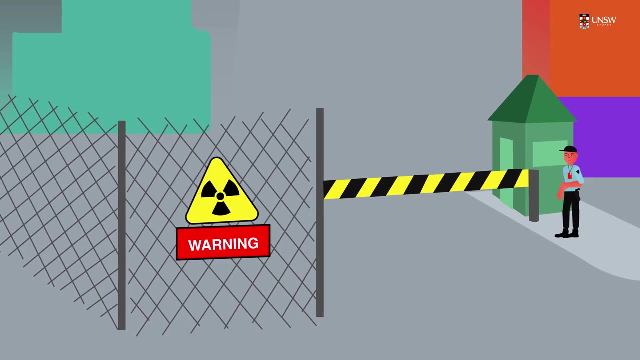 sabotage of safety systems in a nuclear facility. Beyond prevention, nuclear security includes the detection of and the response to criminal or intentional unauthorised acts involving radioactive materials. Nuclear security measures may be physically manifested in the obvious presence of guards with guns and heavy gates that you will see protecting nuclear facilities. And 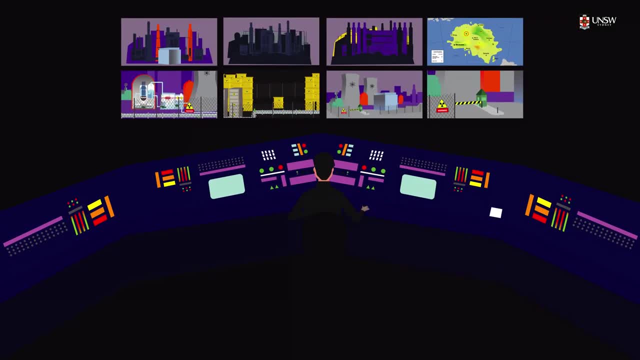 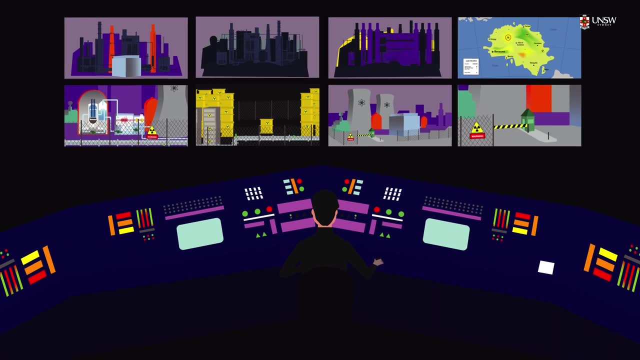 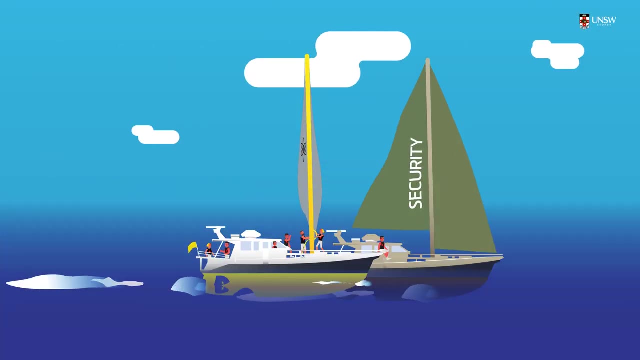 this is one aspect called physical security, But nuclear security also includes the information, electronic and personal security measures that back up the same objectives of prevention, detection and protection. The potentially severe consequences of failures and the need to ensure success in nuclear security means that, just as for nuclear safety, we encounter similar organisational structures: Defence. in depth design principles and legislative and administrative systems governing nuclear security. Nuclear security is the prevention of, detection of and response to criminal or intentional unauthorised acts involving or directly affecting nuclear facilities. The defence of nuclear safety is the safety of the nuclear plants, The use of nuclear 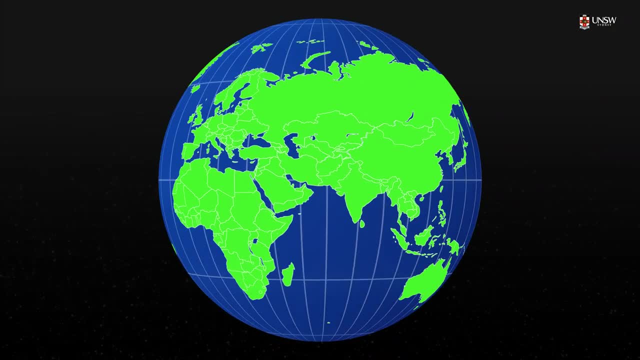 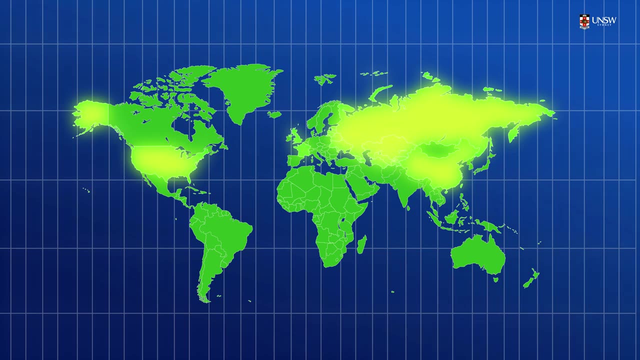 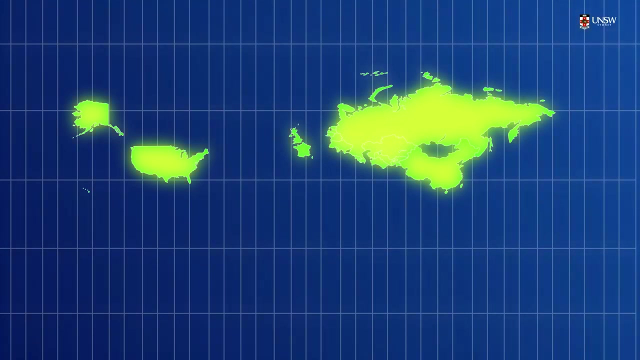 burners is the best way to protect the nuclear material. As an individual person, this is the best way to protect the nuclear material. Nuclear safety requires the experience to be an area of greater concern and stress. as a nuclear safety In the 1950s and the 1960s, the United States, the Soviet Union, France, the United Kingdom. and China repeatedly tested nuclear explosives and became nuclear weapons states. The cost and other barriers to acquiring nuclear weapons was falling for all states. Marshal Peter Louis Shavard, On March 21, 1936, the United States joined the United States and the United States in a nuclear test and test in the United States. Theир aims were to make nuclear 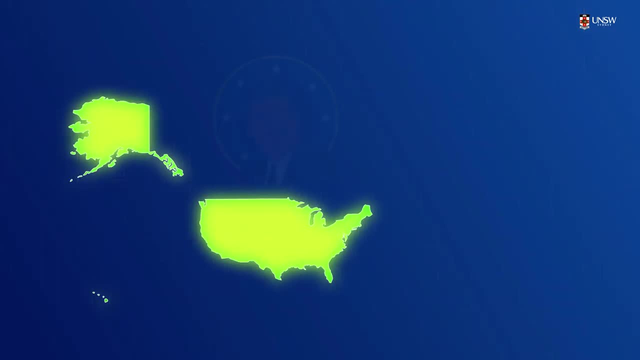 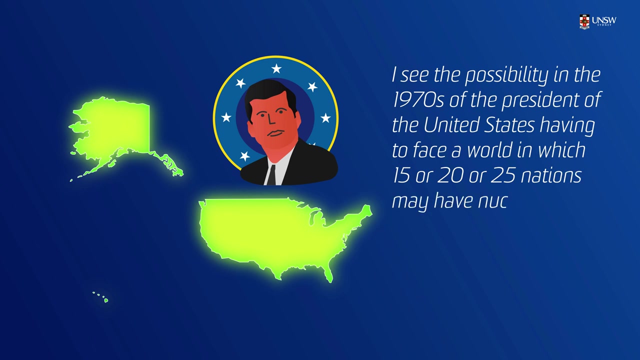 weapons more effective by protecting nuclear weapons. To do so, nuclear ingredients, nuclear weapons- were used. On March 21, 1963, US President John F Kennedy's words reflected the mood when he said: I see the possibility in the 1970s of the President of the United States having to face a world in which 15 or 20 or 25 nations may have nuclear weapons. 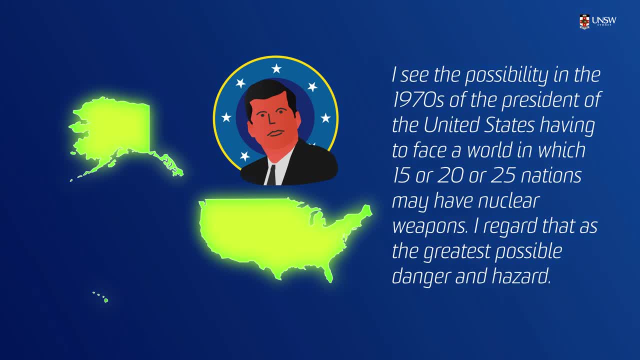 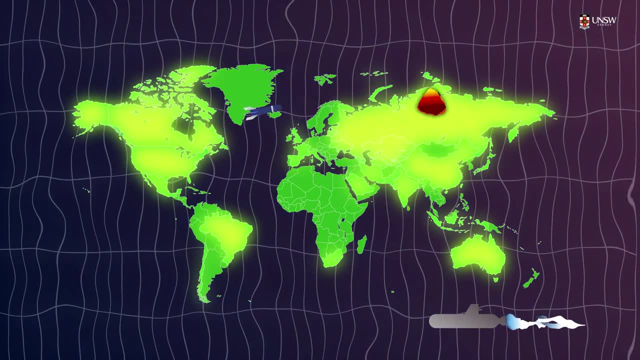 I regard that as the greatest possible danger and hazard. Potentially, more and more states would soon possess nuclear weapons. How could the states of the world reduce the risk that nuclear weapons would be used and reduce the risk of actual nuclear war from spiraling out of control? 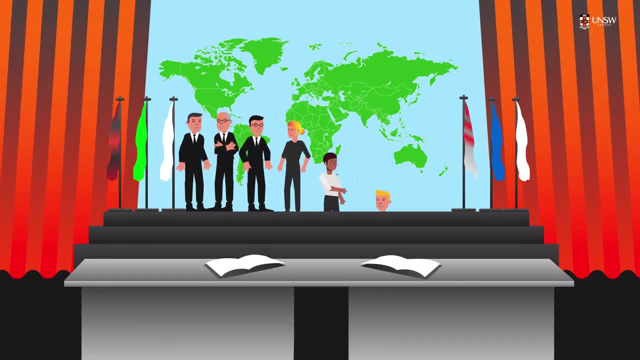 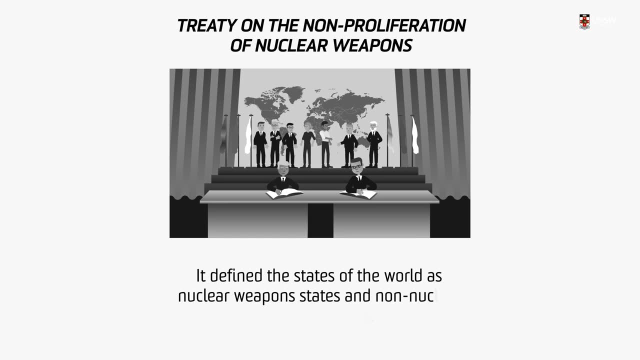 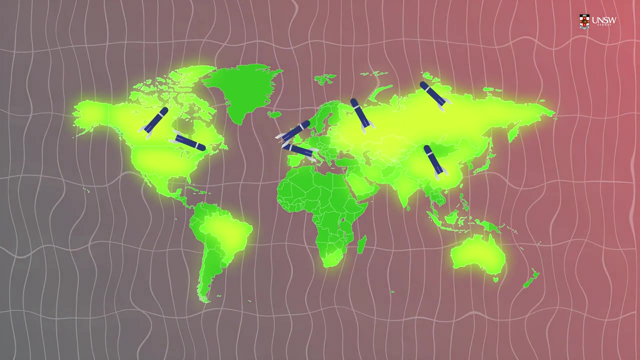 Against this backdrop, the Treaty on the Non-Proliferation of Nuclear Weapons was created. It defines the states of the world as nuclear weapon states and non-nuclear weapon states. The nuclear weapon states agreed to pursue eventual nuclear disarmament. The non-nuclear weapon states agreed to force. 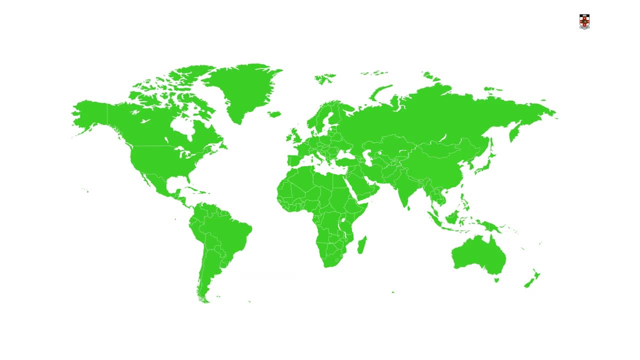 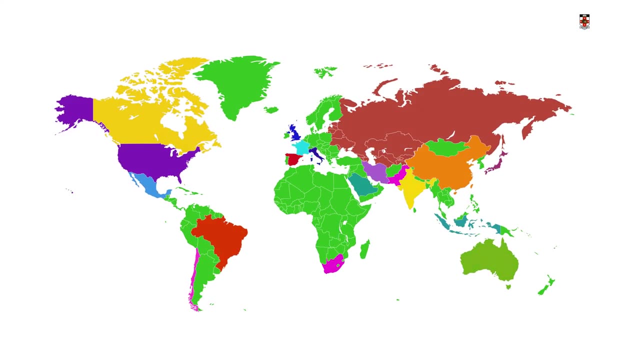 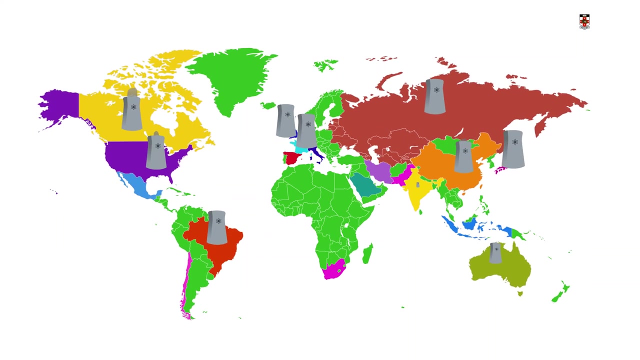 or forego any attempt to develop or acquire nuclear weapons. All signatories are granted an inalienable right to the development of nuclear technologies for peaceful purposes, including the sharing of civil nuclear technologies and helping each other in trade, in advice and in other collaborative work to facilitate peaceful uses. 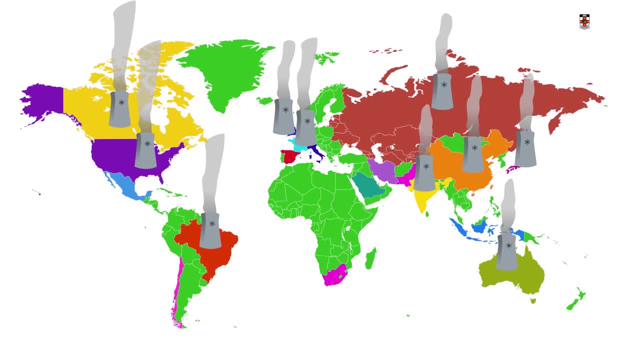 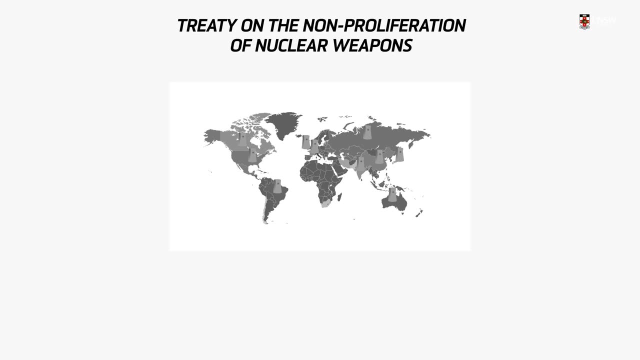 Much of these activities form the work of the International Atomic Energy Agency. The Nuclear Non-Proliferation Treaty entered into force in March 1970 and was indefinitely extended in 1995.. It is one of the most successful arms agreements ever, with near universal membership. 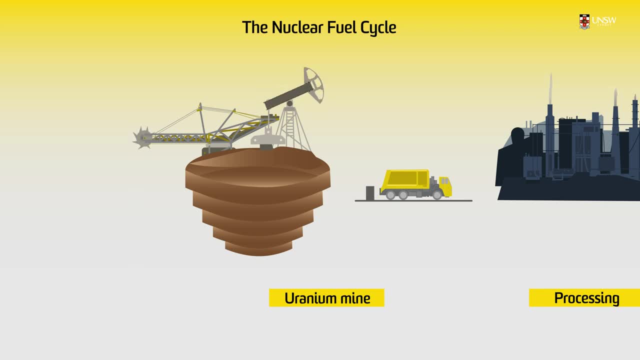 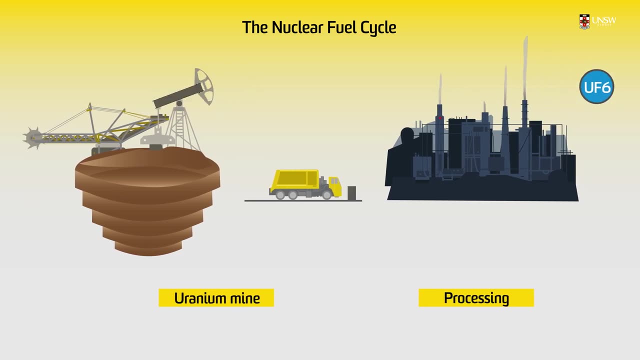 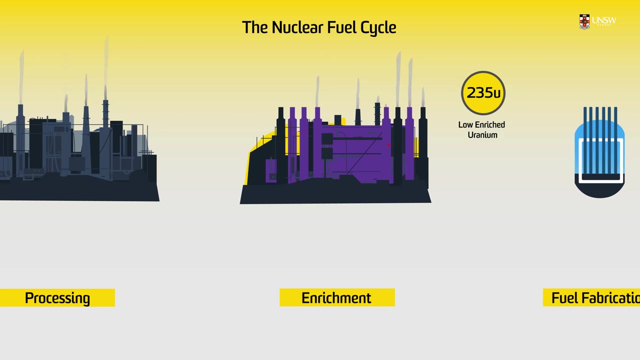 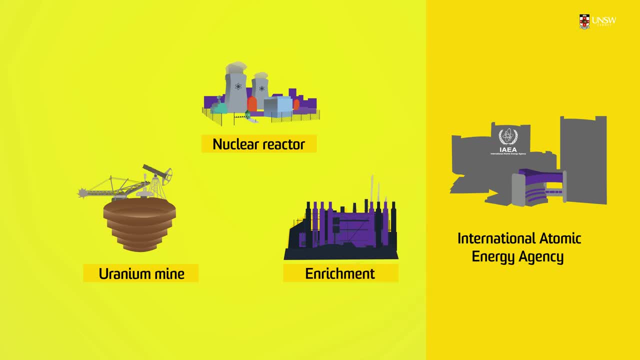 Certain fissionable nuclear materials, such as enriched uranium and plutonium, can be used to produce nuclear weapons. Certain fissionable nuclear materials, such as enriched uranium and plutonium, can be used to produce nuclear weapons. Secondly, the International Atomic Energy Agency will conduct inspections in the nuclear facilities of the State to ensure that what States report is in fact true. 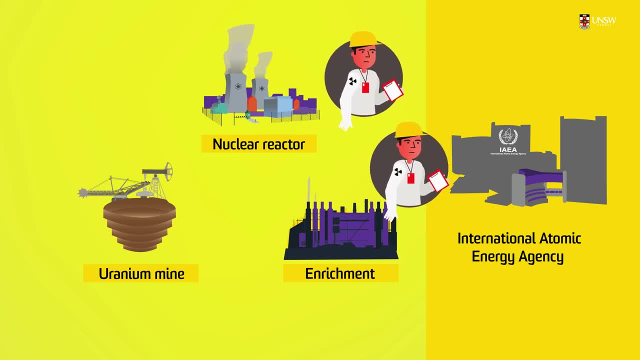 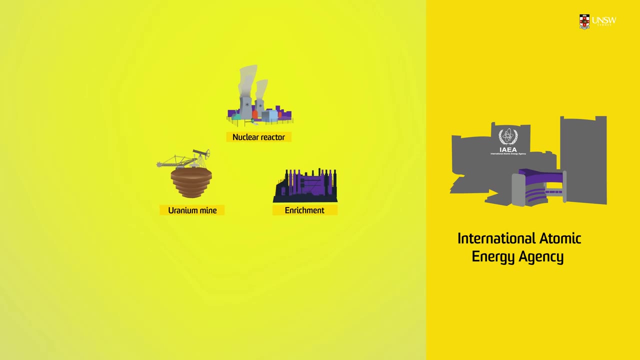 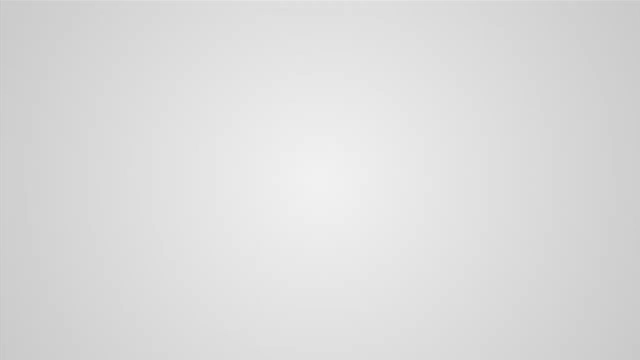 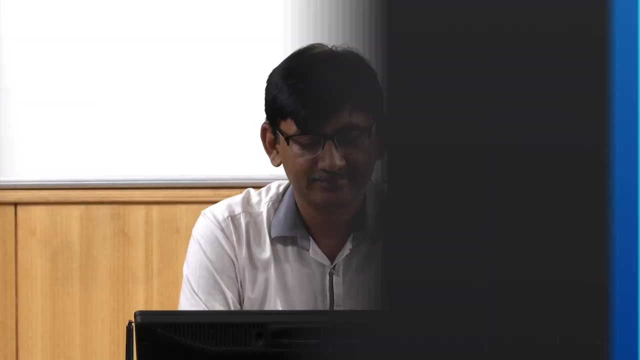 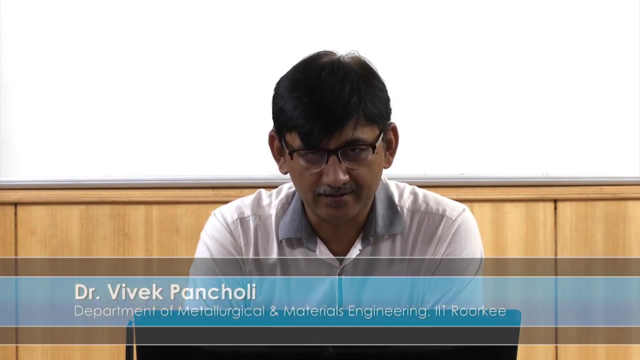 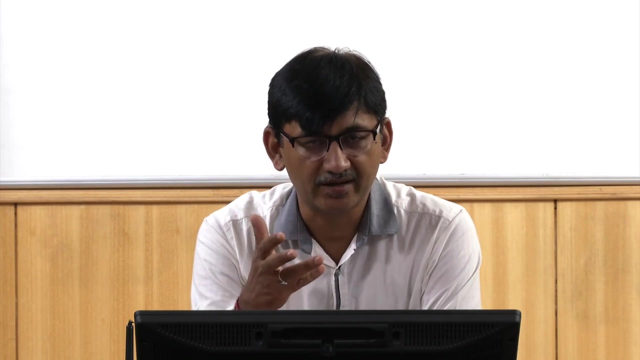 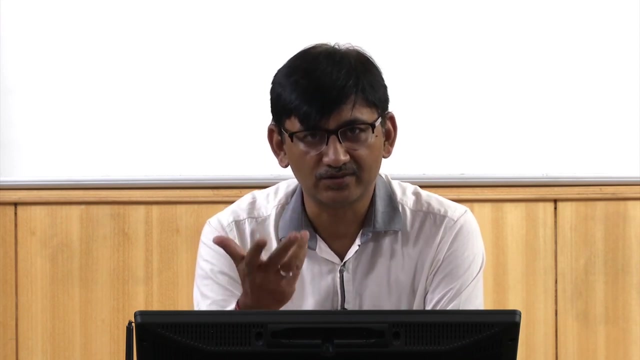 Hello friends, today I am starting with a lecture on Nucleation and Growth. Till now, we discussed all the transformation. first we discussed about the phase diagram and then, using phase diagram, we discussed about the transformation from one phase to another phase, how this transformation is going to take place, and so on, but we did not discuss anything. 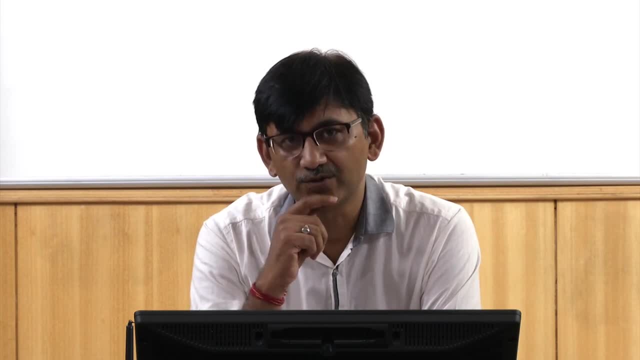 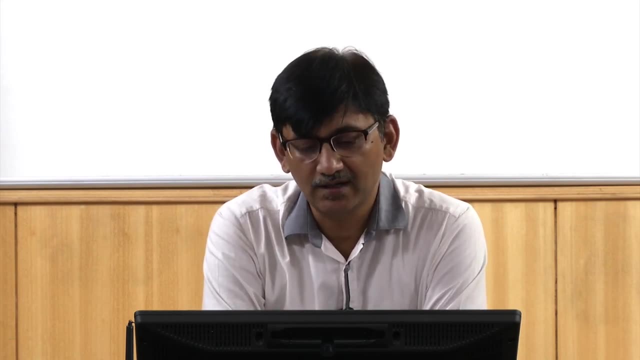 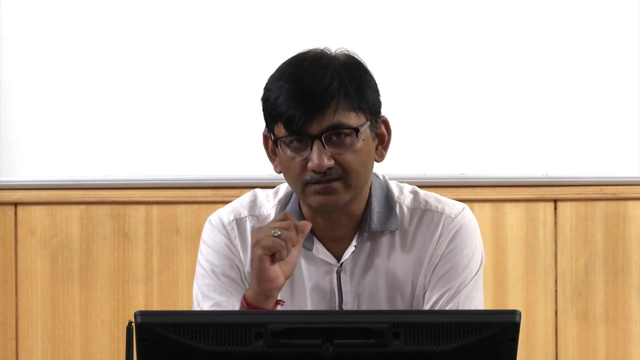 about the rate at which this transformation is going to take place. So now the lectures which we are going to have, Basically we are going to discuss about that, how this transformation is going to take place. So today's course is on nucleation and growth.